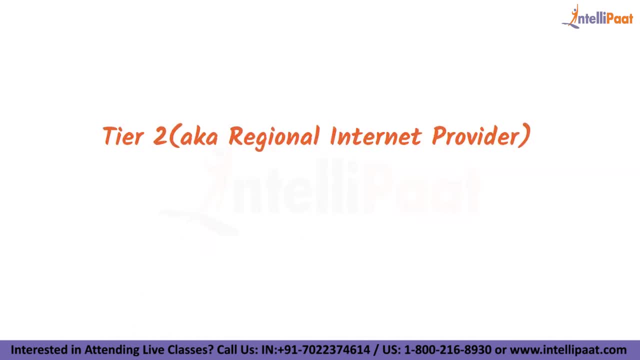 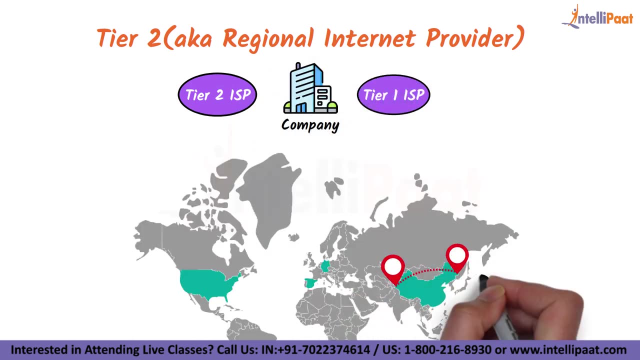 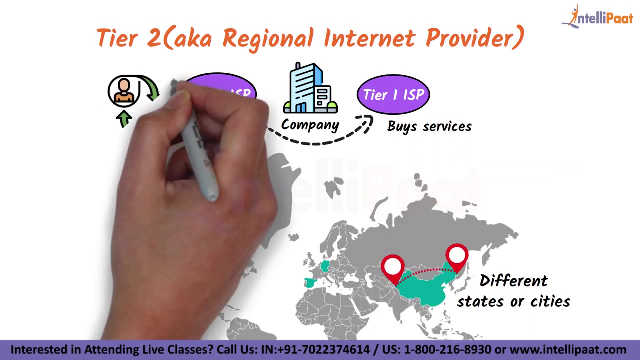 Now let's talk about Tier 2, which is also known as Regional Internet Provider. Tier 2 company is smaller than Tier 1.. This company works to provide internet connection to different states or cities of the country. It means that Tier 2 buys services from Tier 1.. Tier 2 ISPs peer with each other at a 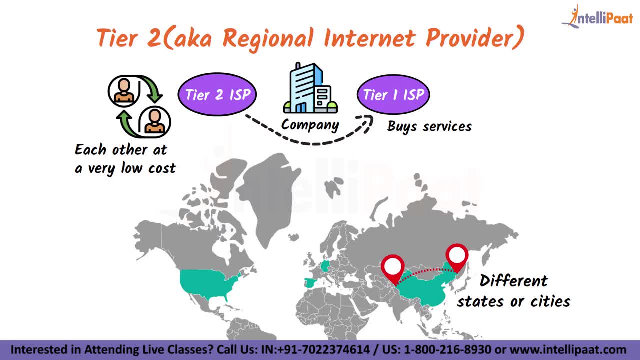 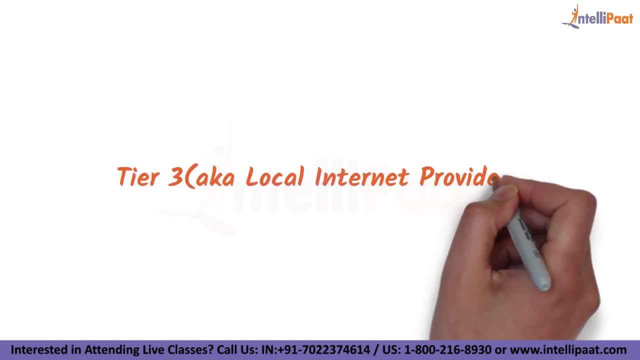 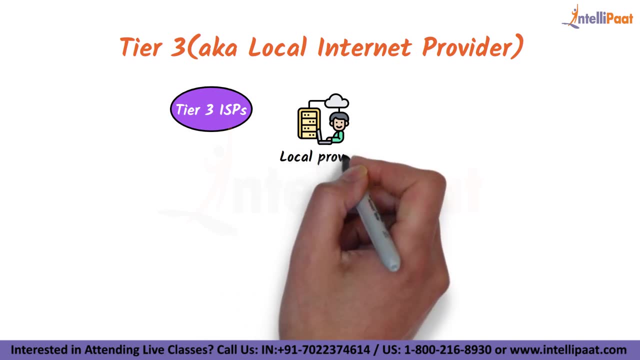 very low cost or no cost at all to expand their global reach Tier 2 companies such as Comcast, Virgin Media, etc. Lastly, we have Tier 3, which is also known as Local Internet Provider. Tier 3 ISPs are most commonly called Local Provider with Metropolitan or National Reach. This is the smallest tier that we have. Tier 2 ISPs are also known as Local Internet Provider. Tier 3 ISPs are most commonly called Local Internet Provider with Metropolitan or National Reach. Tier 3 ISPs are most commonly called Local Internet Provider with Metropolitan or National Reach. It works to provide. 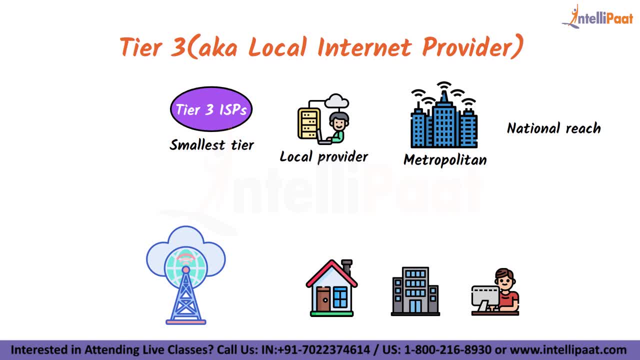 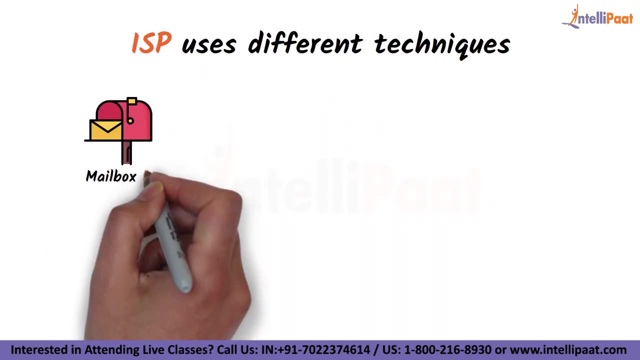 internet services to home companies, offices and block-through routers. That means Tier 3 companies buy internet connection from Tier 2 companies, For example Hathaway Broadband. Now ISP uses different techniques, such as Mailworks, ISP Hosting, ISP Transit, ISP. 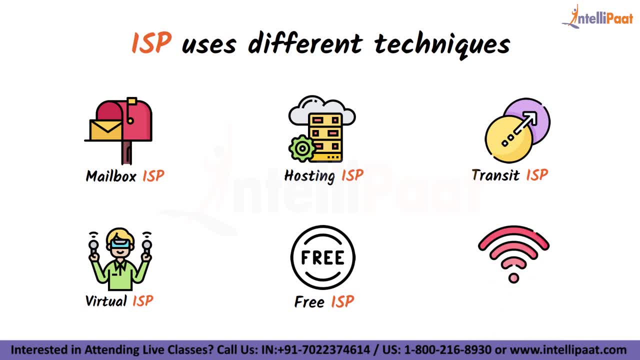 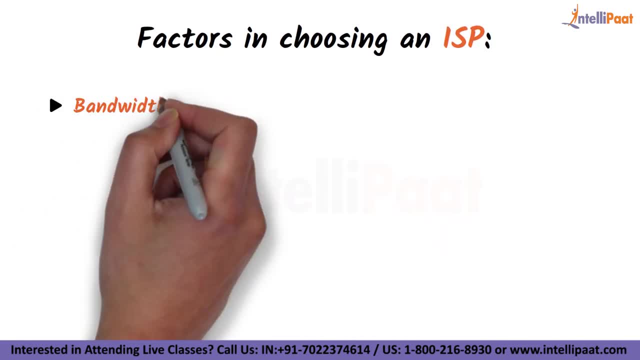 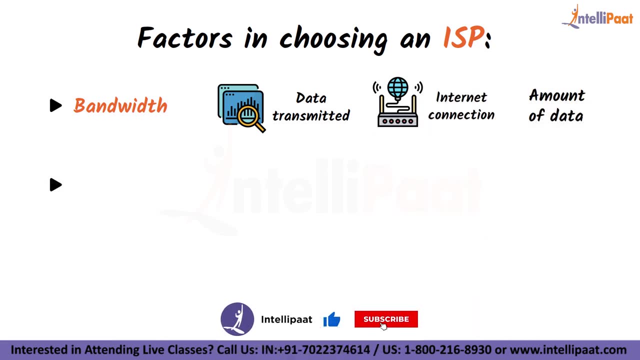 Virtual ISP, Free ISP and Wireless ISP. Now let's take a look at the factors in choosing an ISP. Firstly, we'll talk about bandwidth. The maximum amount of data transmitted over an internet connection is given in an amount of data. Next we have connection stability. 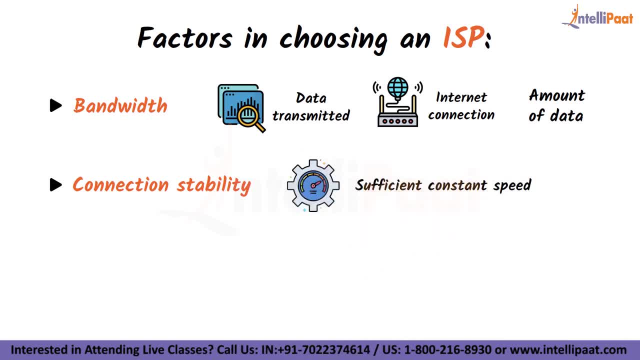 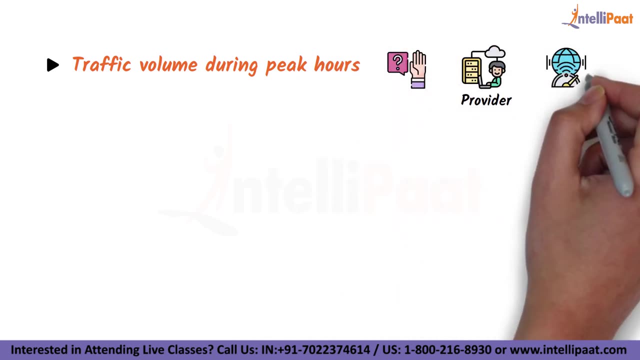 Make sure that they will provide sufficient constant speed. Next up, we have customer volume and traffic. It is very important to check the traffic and how many customers they can have, along with how they are maintained. Next up, we have traffic volume during P-Cars. Ask your provider if they provide you to high speed. 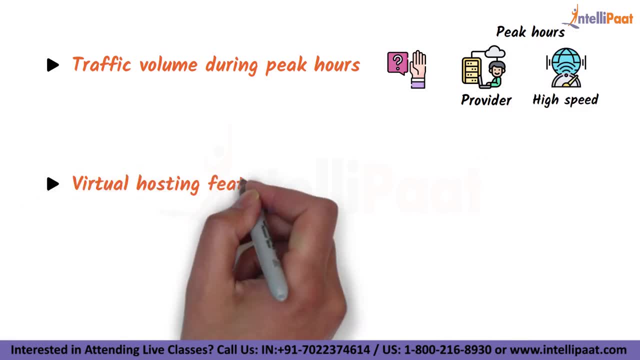 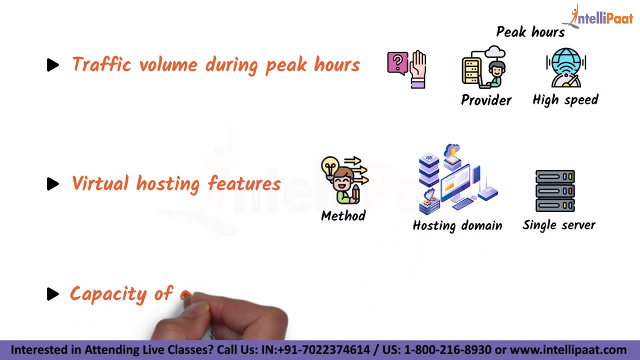 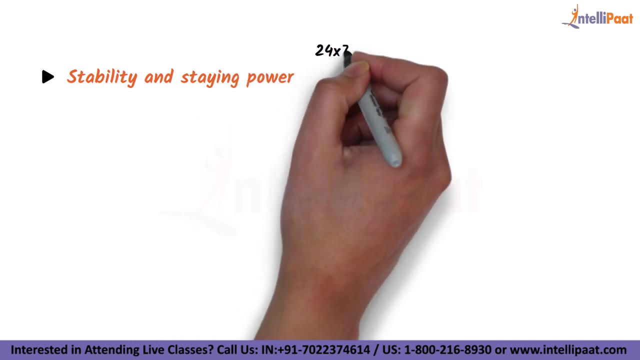 cars. Our next point is virtual hosting features. It is a method for hosting multiple domain names on a single server. Next we'll see capacity of emails box. Compare with others and choose the best one. Next, there is stability and staying power. It should be 24- 7 throughout the year. 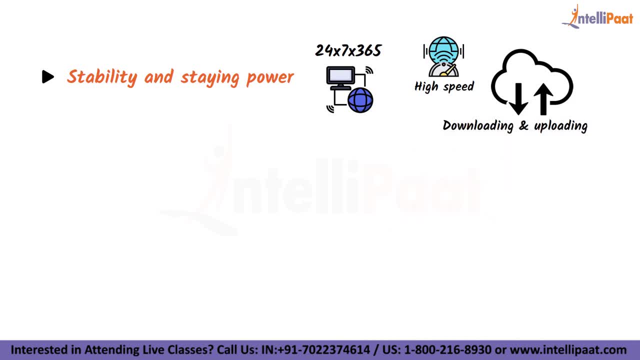 connection with high speed of downloading and uploading. Next, we'll see customer service and local support. Whenever needed assistance, they can resolve your problem quickly, accurately, on a first contact. Lastly, we have price. In order for an ISP to make sense for you, it needs to.